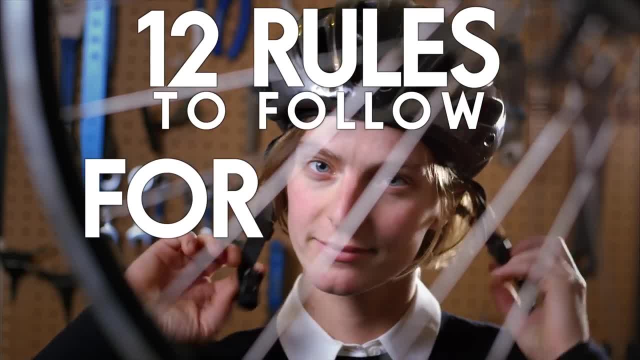 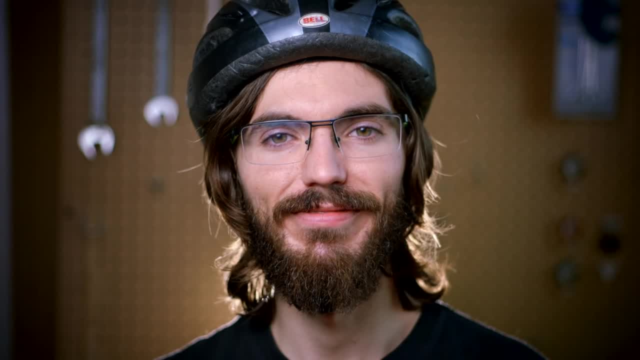 idea. Here are 12 rules to follow for safer biking. Number one: the three-finger rule: Two fingers above your eyebrows and one under the chin. If it's not snug, then it's just a hat. You can do this yourself. 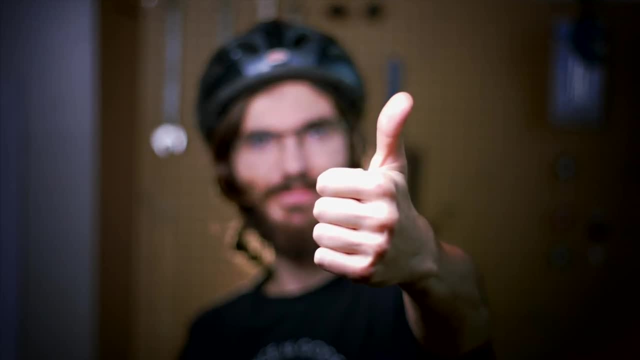 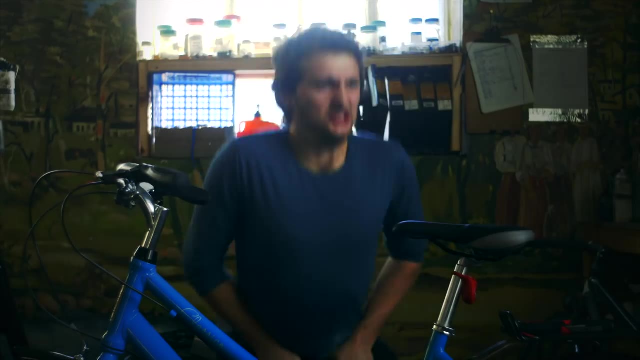 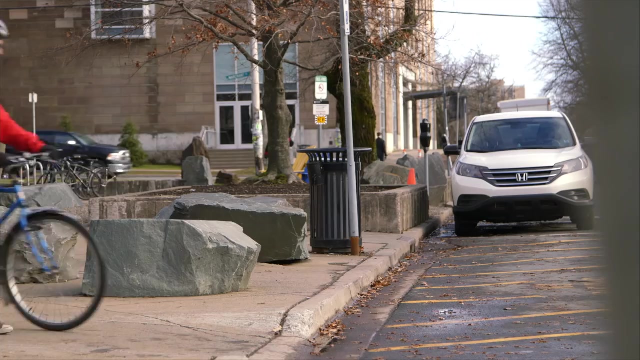 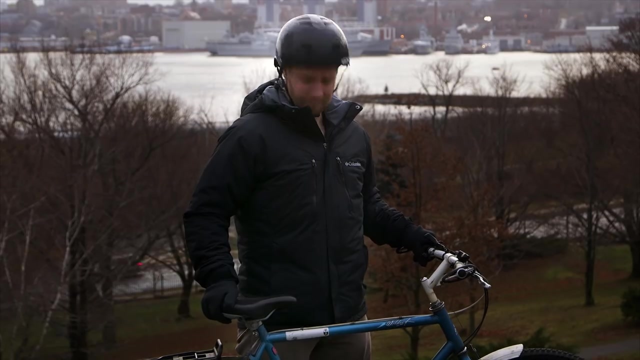 Remember it's the law Wearing a helmet, not putting it on yourself. Numbers two all the way through: six Checks to do before you ride: A for air, B for brakes, C for chain, Quick for quick release, Locked and it keeps your tire on. That's important Check. 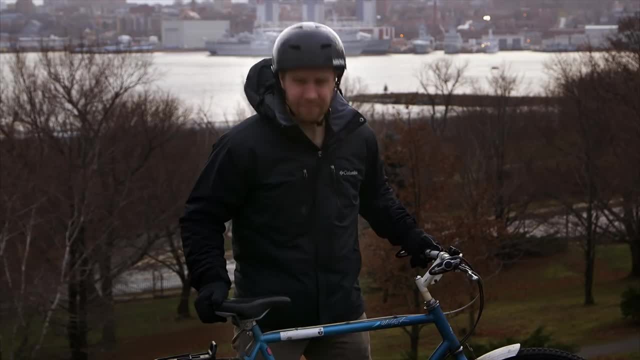 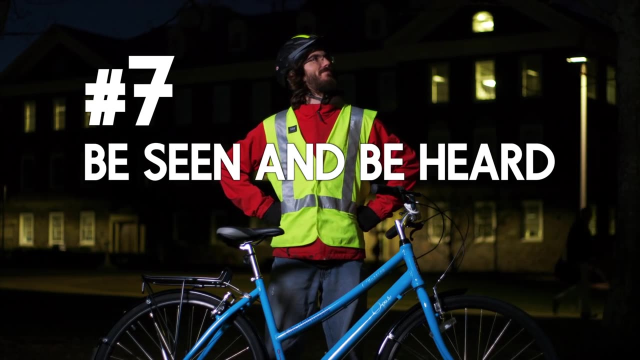 for check. Pick up and drop your bike. Nothing fell off. You're probably good Number seven. be seen and be heard. The law states you have to have a bell or a horn And you need to have a white light in front and a red light in rear. If it. 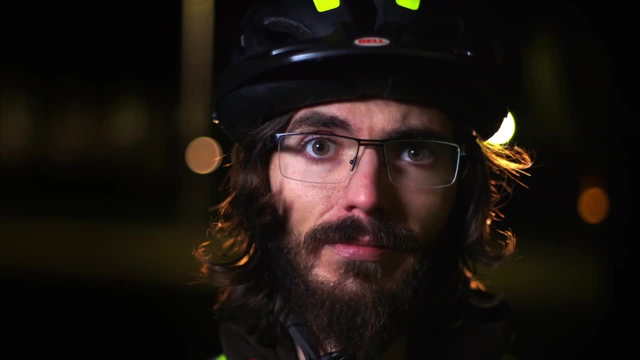 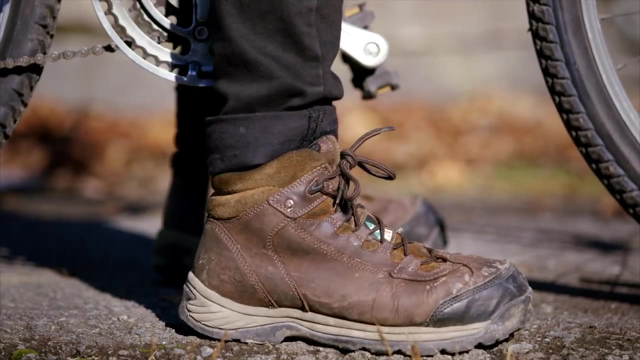 flashes all the better. Like Rudolph- Yes, he's real. What Number eight? seat height and frame. Frame size is important: Feet on the ground and a few inches between you and the frame. If it doesn't fit, then return your bike. I. 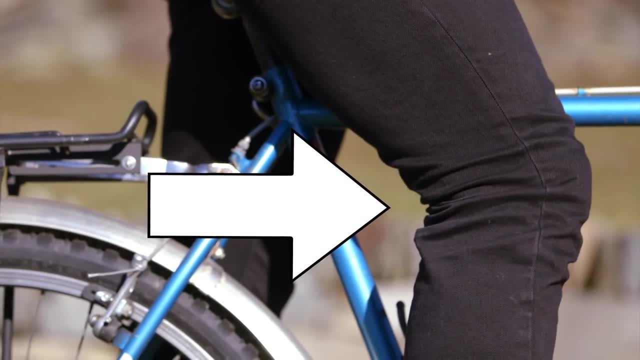 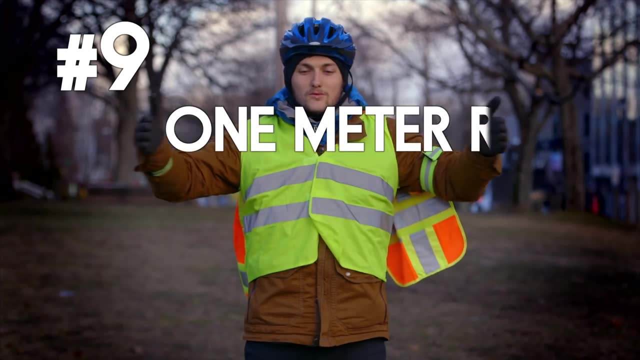 guess Your seat should be high enough that you have a slight bend in the knee at the bottom pedal position. You don't have to ride like this anymore. Number nine: the one-meter rule. By law, a motor vehicle cannot pass a bike on the. 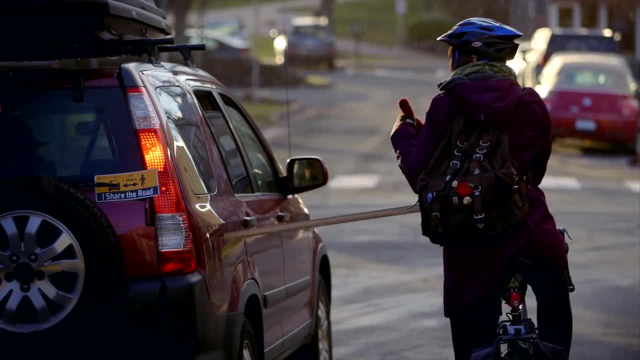 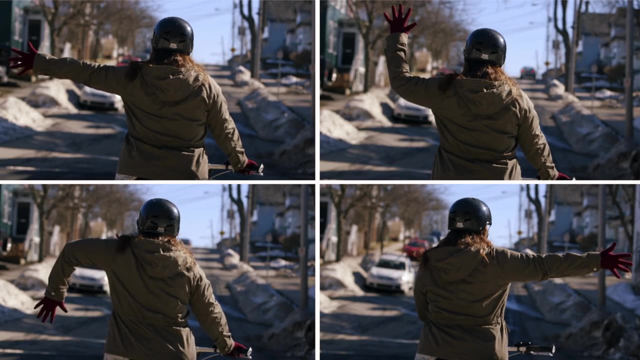 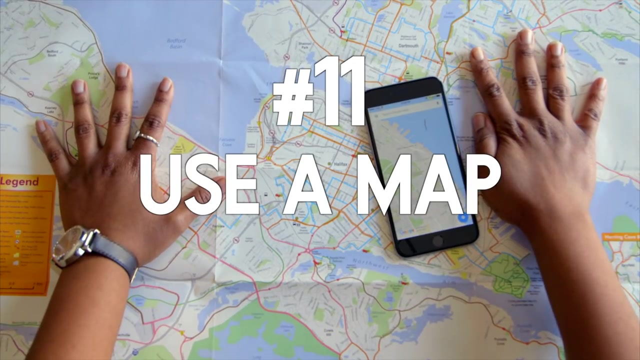 road without one meter between them. Keep this in mind. Number ten: signal signaling. Do this or this for right turns, Do this for left turns, Do this to stop. There are only four signals. Number eleven: use a map. Plan a route with bike. 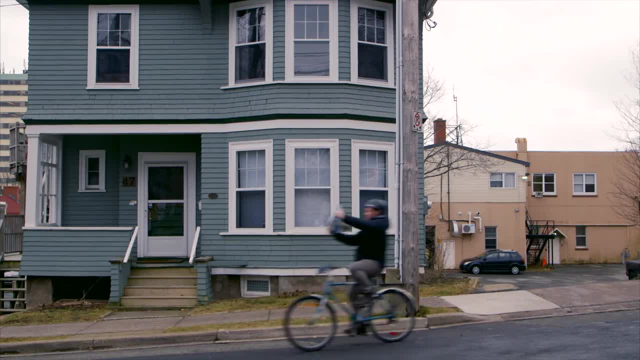 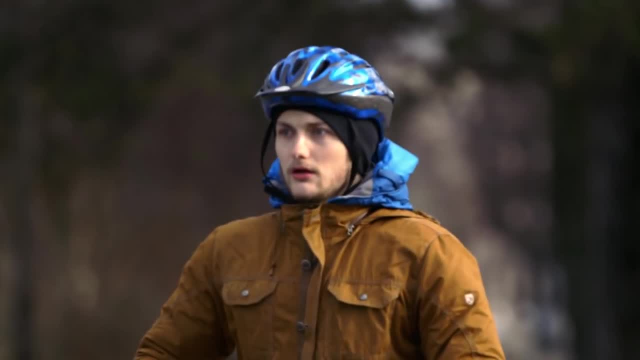 lanes, paths and side roads, And leave your map at home. Number twelve intersection tips: Don't mouse away, Don't be scared, Find a space where you are visible to cars and obey all traffic signals. And if you're ever uncomfortable, 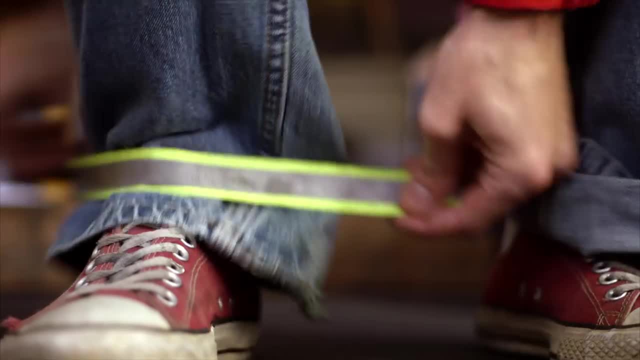 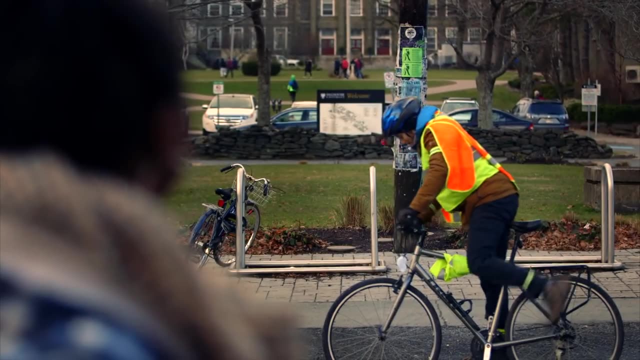 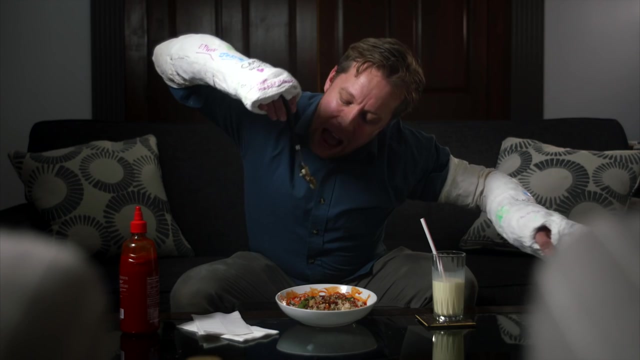 you can always walk on the crosswalk. Follow these twelve rules and you'll be safer, more efficient, responsible and stylish. I respect your wardrobe choices. You can keep yourself and others safer. Make the right choices. You won't regret it.